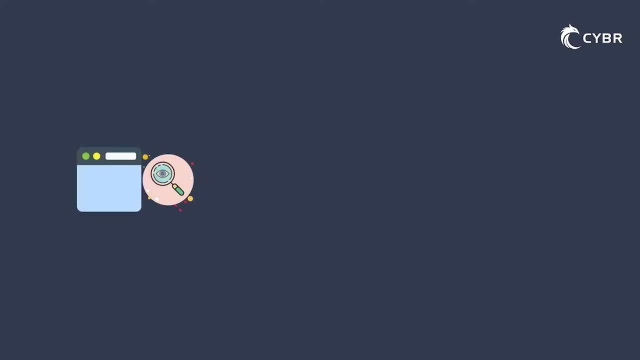 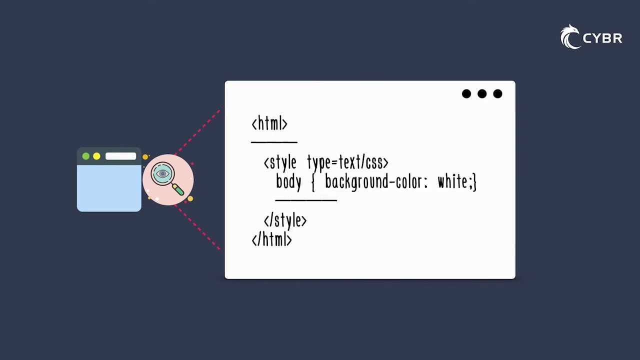 Let's say that you have a static website that's made of only HTML and CSS, And when you visit the website, the browser renders that HTML and CSS and that's what you see on your screen. But nowadays, most websites also include dynamic elements, For example: 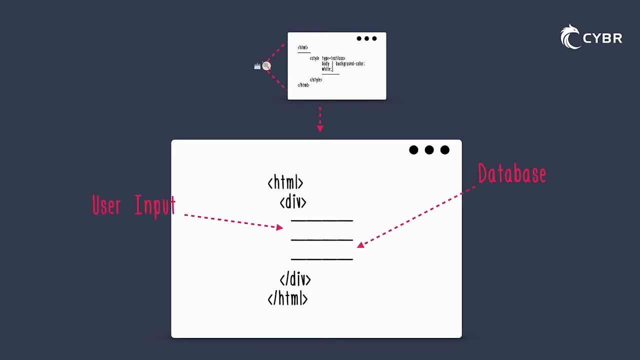 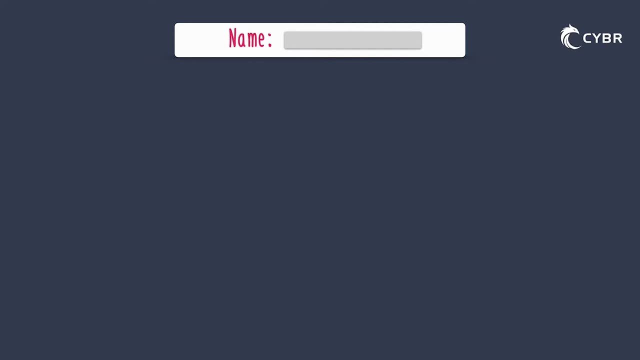 data gets pulled from a database where it asks for user input and uses that user input to do something. So if we visualize that, you might see an input form where the user submits information and the application sends that information to another page via the URL. 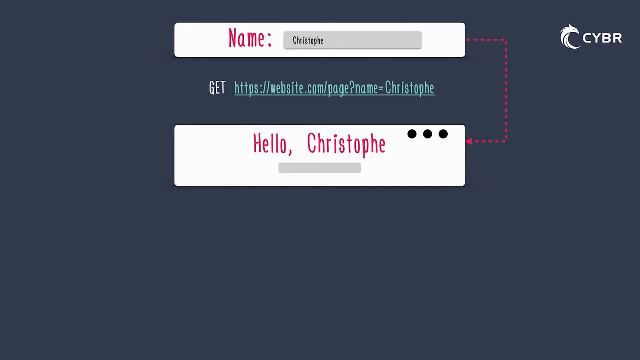 That other page grabs that URL and parses the information in it to grab what the user submitted. Now, let's say that this information is then used to populate an HTML field on the page, in which case it grabs that data from the URL, parses it and then outputs. 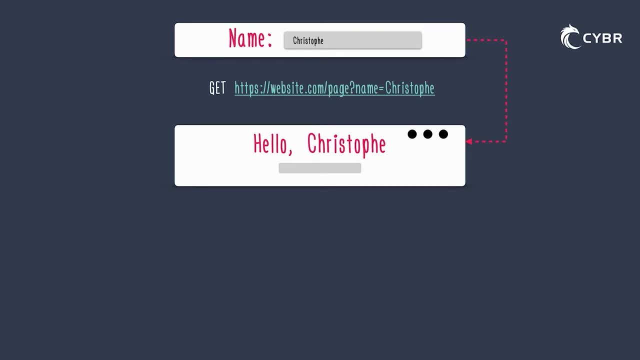 it in the HTML of the page, essentially allowing the user to modify that page. Now, if we put our developer hats on for a minute and we pretend that we have done a direct access to modify the code on this page, we could say that you know what I. 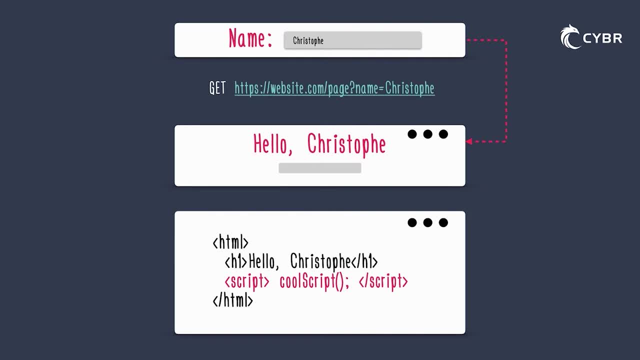 need to add a script to this page in order to enhance functionality. Usually, to follow best practices, we'd either add the script in the header or the footer of the page, but technically speaking, the script can be added anywhere in this page. In fact, we could add: 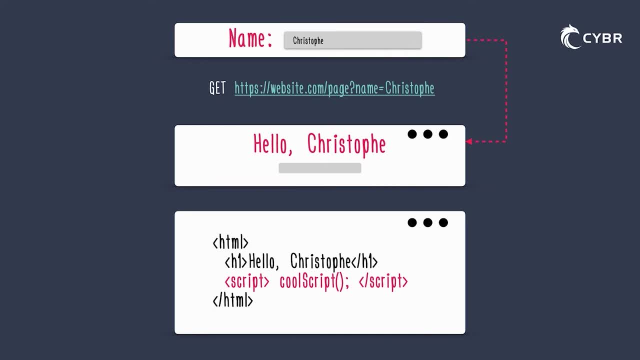 our script right here and the browser would load it when the webpage gets rendered. This means that under the right circumstances, an attacker can abuse that to send a script payload via the URL. So if we want to do this, we could add a script to the URL and then modify the application. 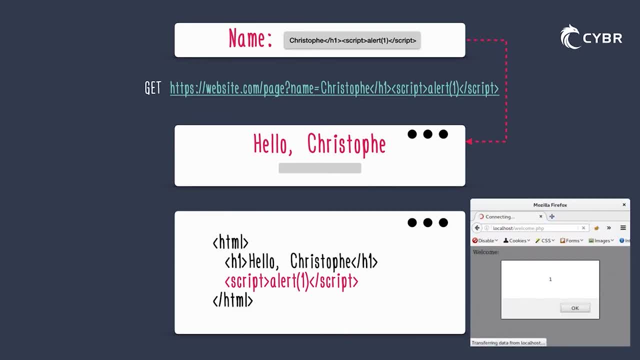 to do something that it wasn't intended to do. In other words, the attacker could inject a malicious script which would then get loaded by the browser, since the browser thinks that it's part of the webpage and that it needs to load the script for that webpage to function. 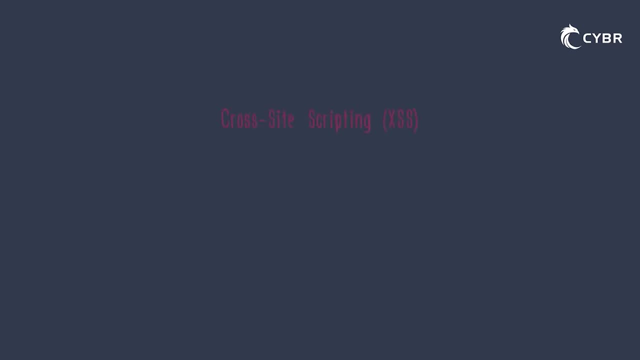 properly Enter cross-site scripting. Cross-site scripting, aka XSS, is a type of injection attack where malicious scripts are injected in trusted websites and executed by the user. This is a type of injection attack where malicious scripts are injected in trusted websites and executed by the user's browser. A simple, supposedly safe website with users and an attacker finds a way to exploit that website in order to send malicious code to one or more of those users. That malicious code is generally in the form of browser-side scripts, so really nothing crazy or fancy. 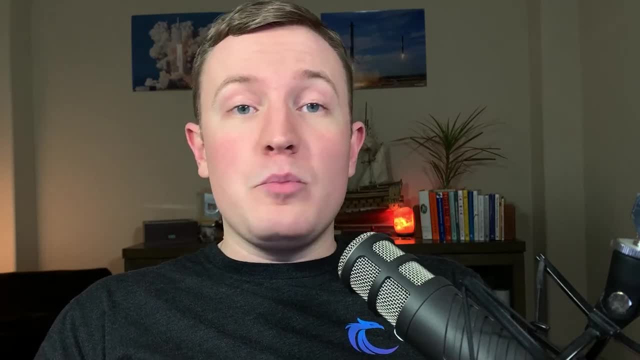 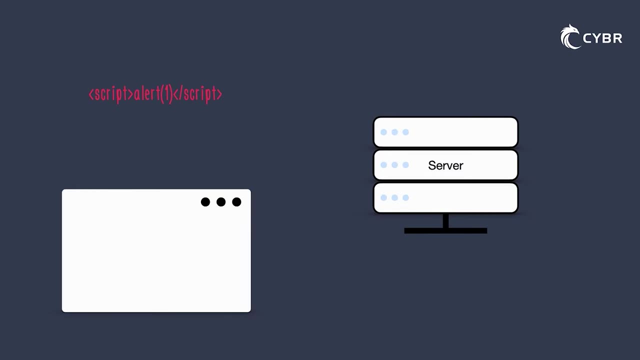 at all, literally what everyone with internet access is able to create. An attacker finds a way to take their malicious code and infect the HTML document without causing the web server itself to be infected. Instead, it uses the server as a vector to present malicious content back to the user, either instantly from the request, which is called. 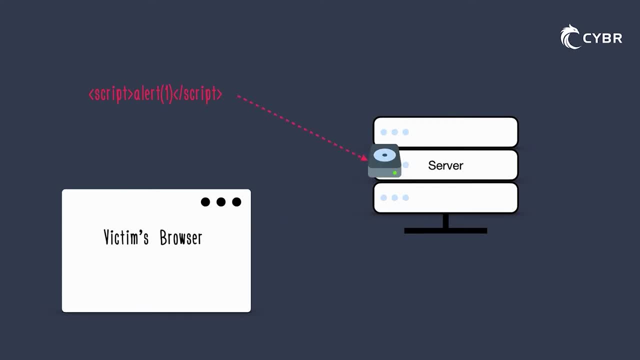 a reflected attack or delayed through storage and retrieval, which is called a stored or persisted attack. But again, and to clarify, even when I say that the malicious code is stored and retrieved at a later time, I don't mean that the server itself is infected with malicious code. The 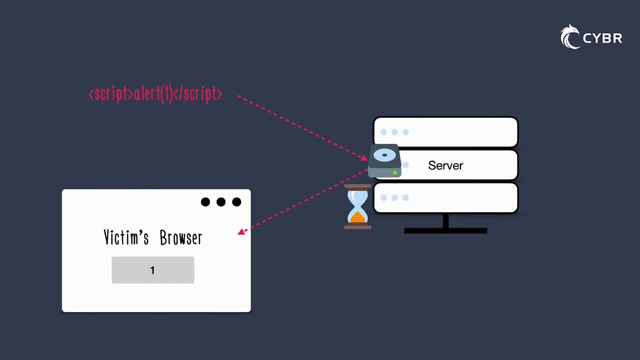 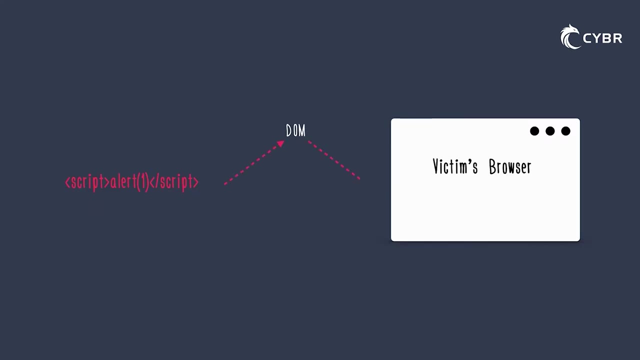 malicious code only gets executed through the user's browser when that user visits a web page that fetches the stored code. So the core application remains completely unaltered, but it can be made to serve malicious content to its clients With a third type, DOM-based. 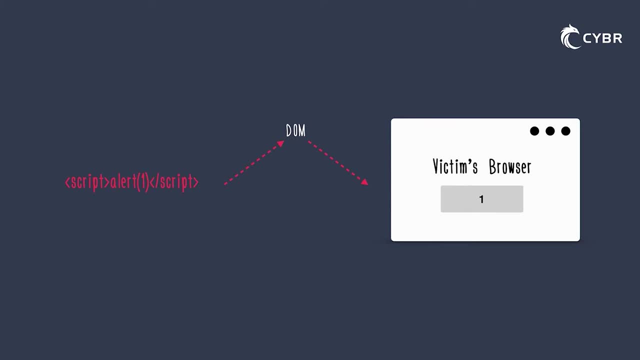 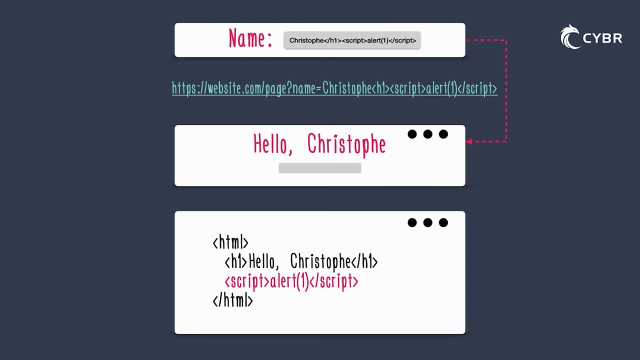 the payload technically never even has to reach the servers at all. So then, when is cross-site scripting possible? What causes the vulnerability and how do people exploit that vulnerability? Like other types of web-based injection attacks, cross-site scripting attacks are possible when an application uses input from 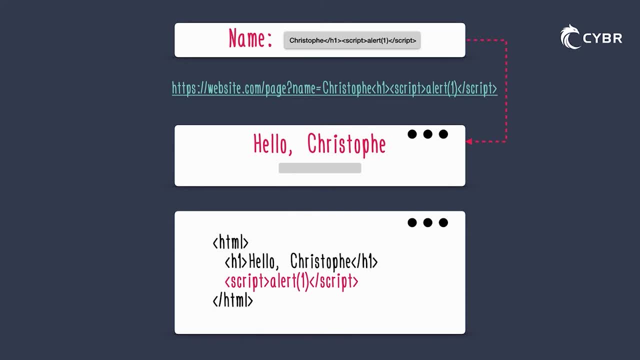 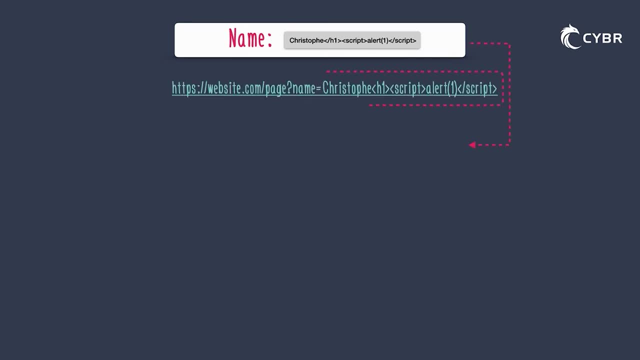 a user within the output that it generates without properly validating or encoding that data. And if you're not familiar with the term encoding, it simply means converting data or a sequence of characters into a specified format to securely process that data, And validating refers to 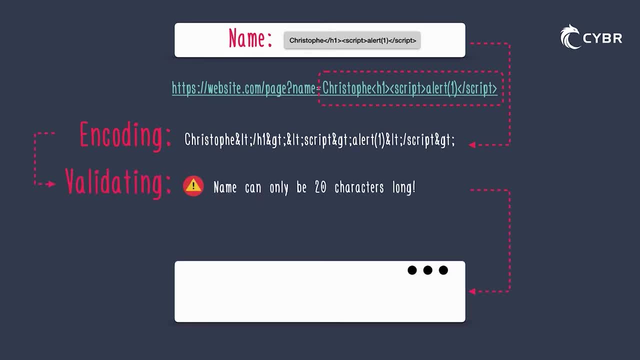 verifying that the data is what you expected. We'll definitely be talking a lot more about encoding and validation in the defense section of this course, but I did want to make sure that you weren't confused by those terms In any case, since we were talking about the application grabbing input from a user and then outputting. 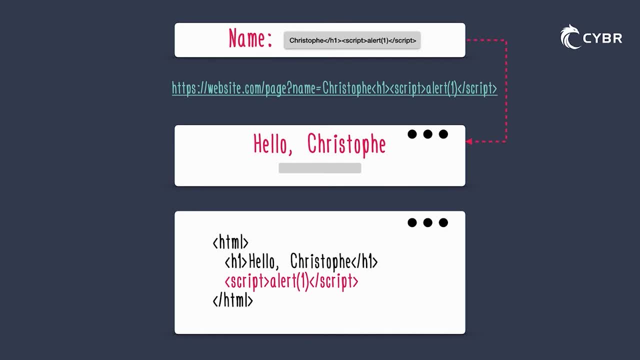 that information. the page is only reflecting back what was submitted in a request, but the content of that request might have characters that break out of the ordinary and expected text content and instead introduce HTML or JavaScript content that the developer did not intend for and that the application did not expect. 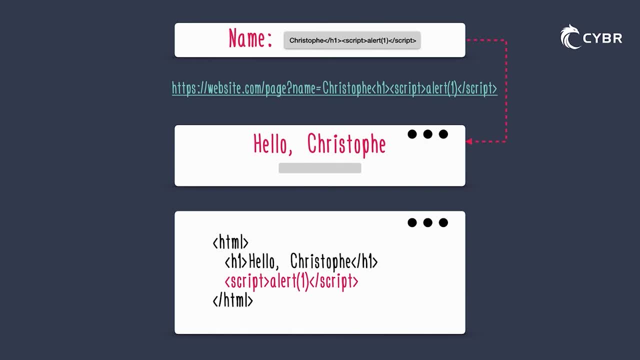 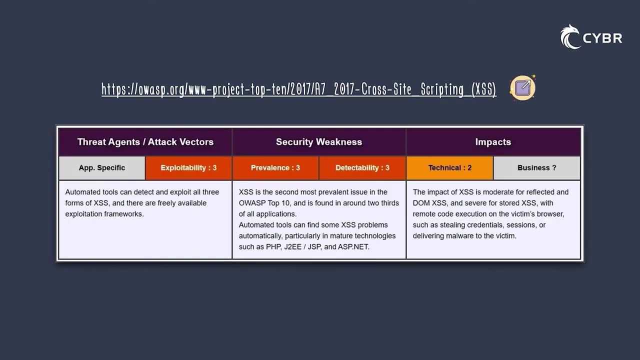 The bad news is that modern browsers are getting smarter and smarter and they now include a lot of defenses out of the box to prevent successful XSS attacks. The bad news is that these browser security controls don't prevent all XSS attacks And while they're definitely not as common as they 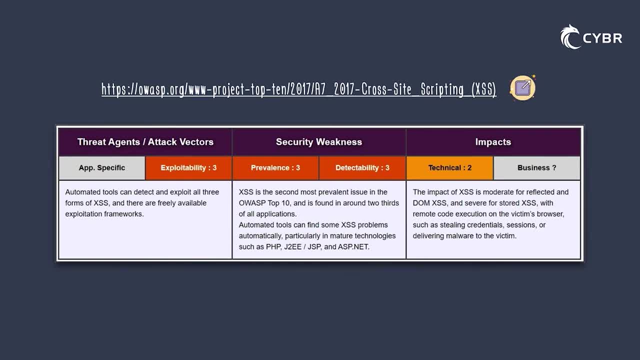 used to be, they're still found in the real world and they're one of the most commonly attempted attacks on applications. In fact, they're listed as one of the second most prevalent issue in the OWASP Top 10, with an exploitability prevalence and detectability of the OSP top 10.. And that's. what we're going to talk about in this video. But before we get started, let's take a look at some of the most common attacks in the OSP top 10.. The OSP top 10 is one of the most common attacks in the OSP top 10.. 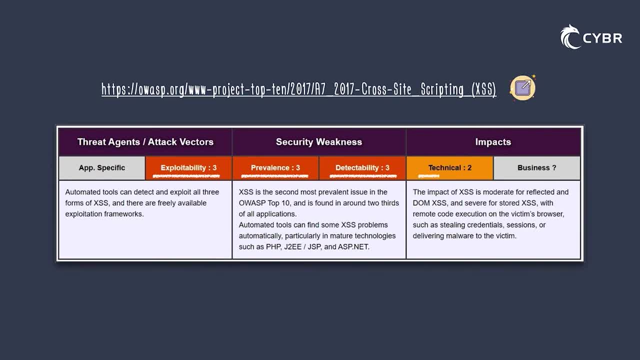 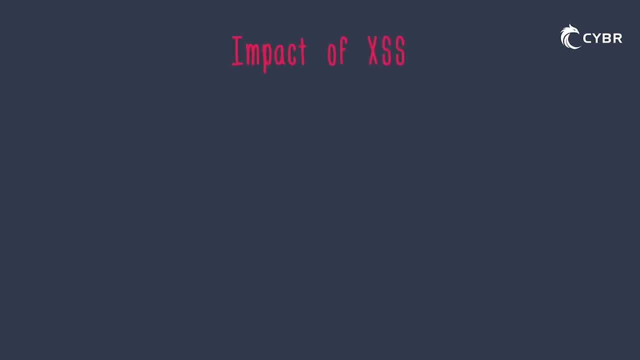 and detectability rating of 3 and a technical impact rating of 2, since some of the XSS attacks will have much less severe impacts than others. Successful exploitation of XSS can do a lot of damage If an attacker is able to inject malicious scripts into a web application. 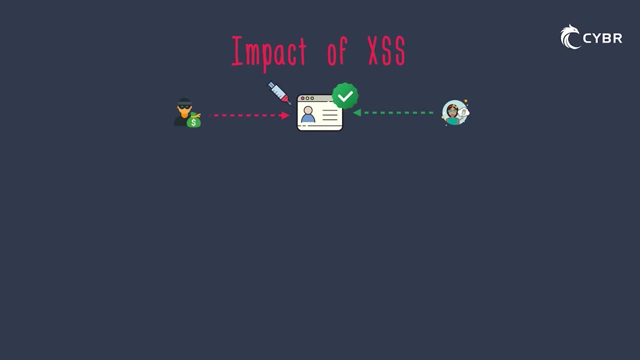 then the browser may end up believing that the script comes from a trusted source And it will let that script access all kinds of information, like cookies, by using documentcookie, session tokens or other sensitive information stored in the browser and used with the site. to number one. 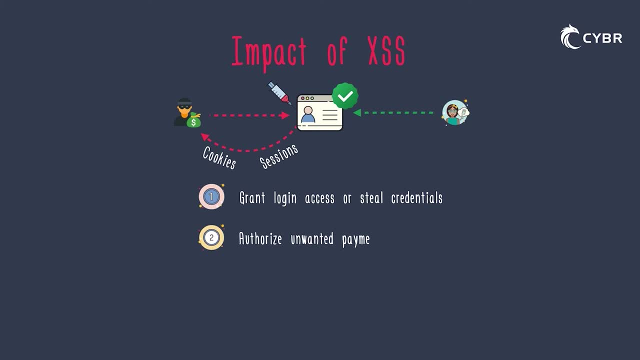 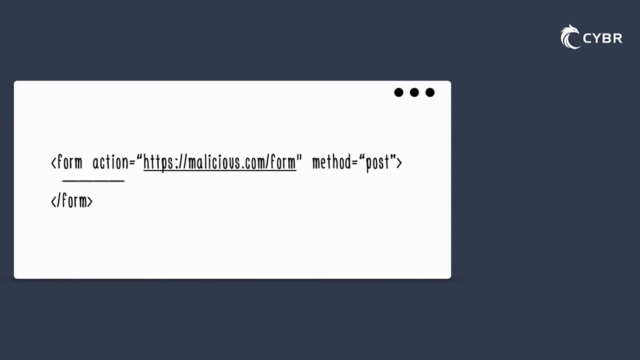 grant login access or steal credentials, authorize unwanted payments, redirect users to a lookalike website and a whole lot more. Some scripts could even potentially rewrite the HTML on the page, changing the appearance of the website and causing you to perform actions that you may. 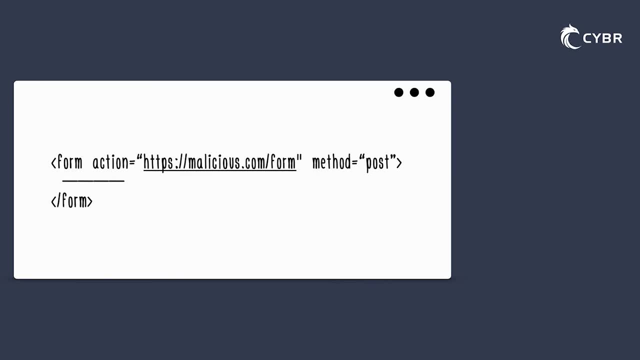 not otherwise take or sending your private information to another server without you realizing it. For example, an attacker could insert a fake login form into an existing page and set the form's action attribute to target their own server and therefore trick the user into submitting. 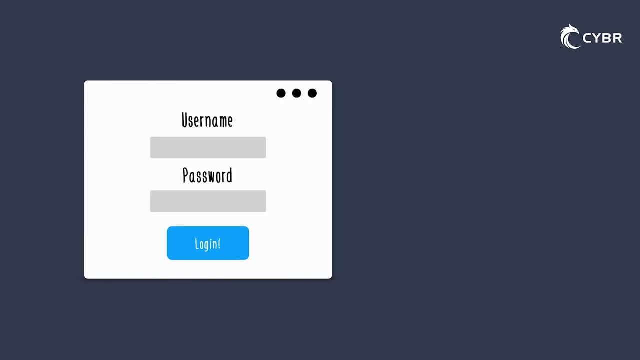 sensitive information without even realizing it, And apart from the information that we've already talked about, an attacker could also register and send a user's keystrokes to their own server by adding what's called an event listener, with the add event listener method, potentially recording sensitive information like passwords and credit card numbers. 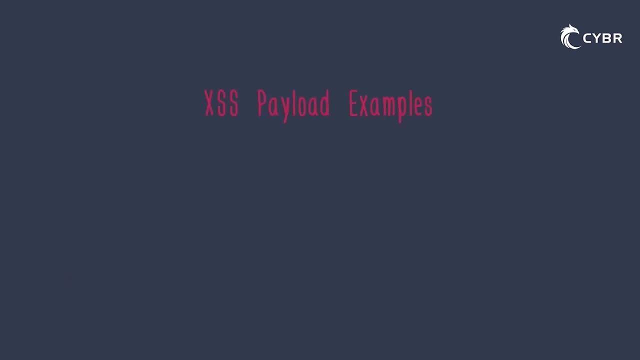 So let's take a look at some examples of basic XSS attack scripts so that we can illustrate the concepts that we've been talking about. One of the most common examples you'll see, and also, frankly, one of the least realistic or practical examples, is the alert injection, which looks like this: 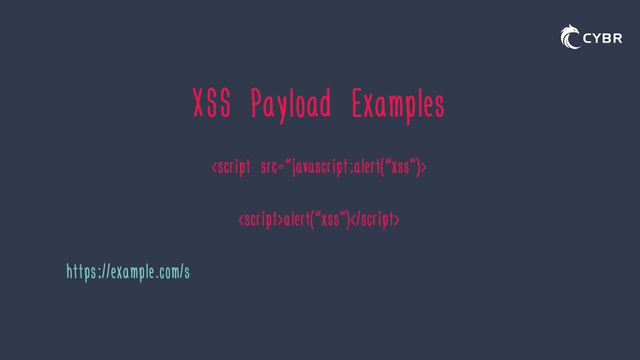 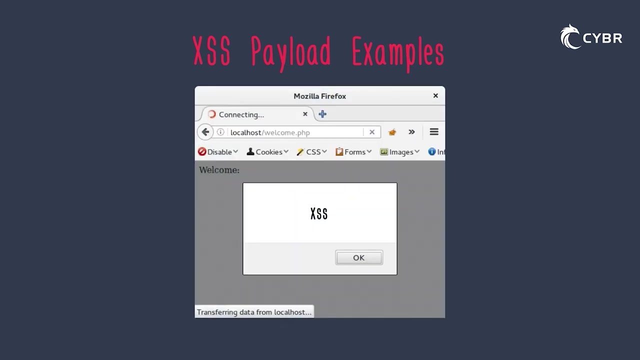 And this alert injection could happen via a URL like this, or it could be injected in vulnerable input fields. All this would do is create one of those annoying alert boxes that just writes out XSS, but this is meant as a proof of concept for the user to be able to use it. So if you're.